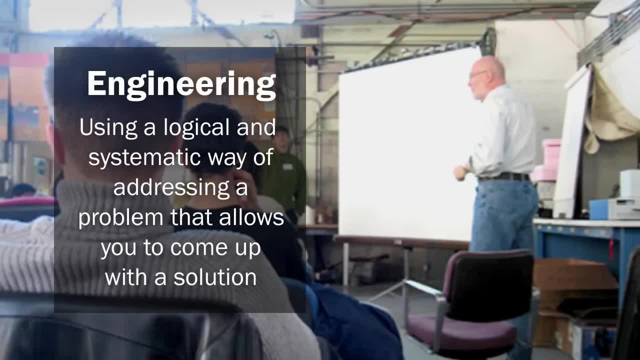 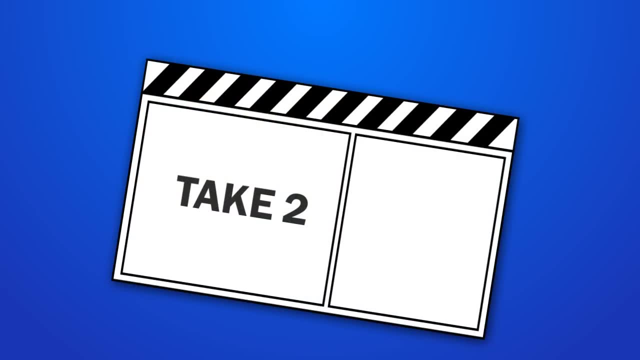 Engineering means using a logical and systematic way of addressing a problem that allows you to come up with a solution. But it's not magic, It's logic. Okay, problem solving. take two: We start with a problem. Let's say we need to get from here to here. 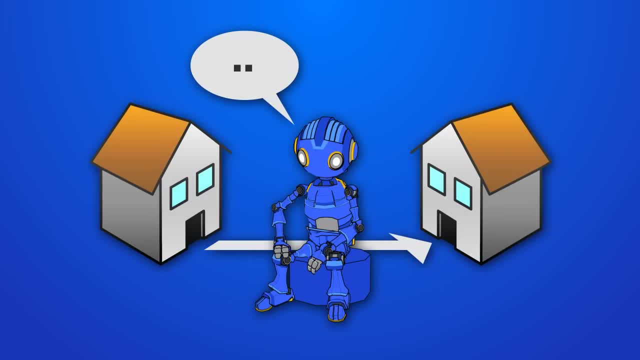 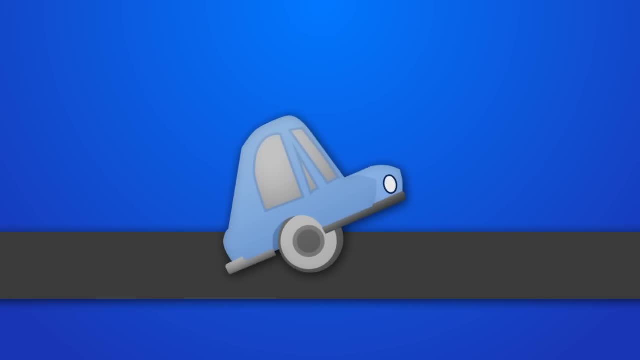 Since we can't use magic, We'll just have to sit down and think up an idea And then we build the thing we thought of And voila- solution. What the heck Did you guys even test that thing? Okay, third, try's the charm, right? 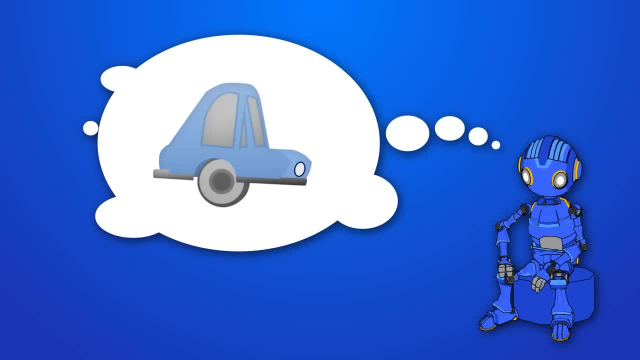 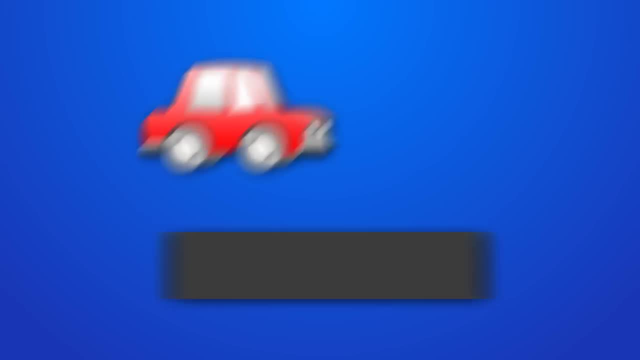 Start with a problem, Then, instead of taking the first idea that pops into our heads, let's get a bunch of ideas, collect them and pick the best one. Now let's build based on that idea And test the product to make sure it actually works. 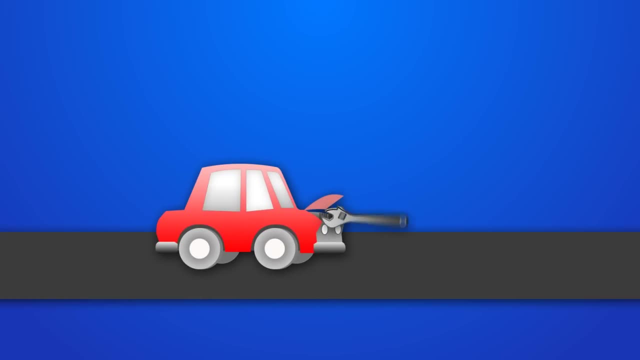 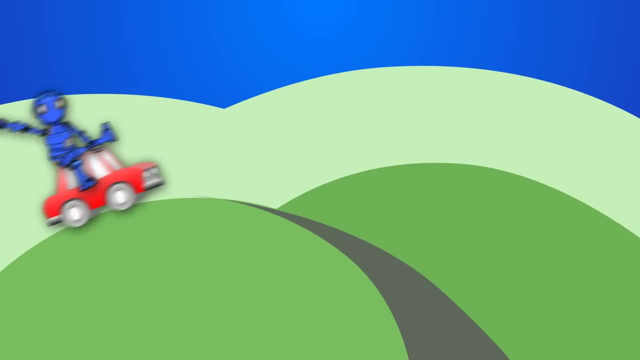 Okay, let's go. If something doesn't work quite right, let's change the design slightly to fix the problem and try again And repeat that until everything works. Now we take our solution and sell it to uh hi there. Well, it looks like we may have another problem or two. 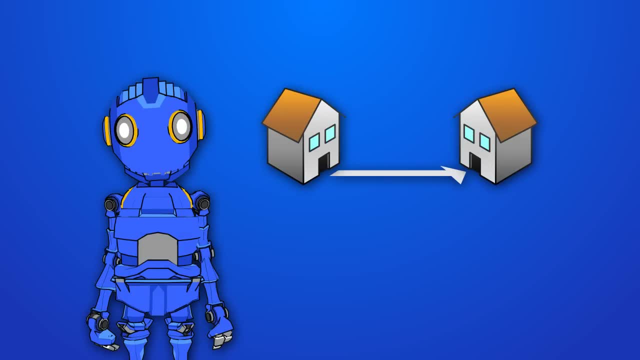 Let's add in here: when you start with a problem, you should probably do a bit of research on it first. Clearly, we didn't quite understand just who is going to be using it. Let's add in here: when you start with a problem, you should probably do a bit of research on. 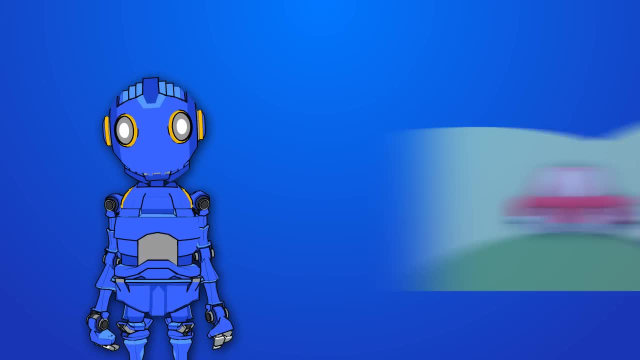 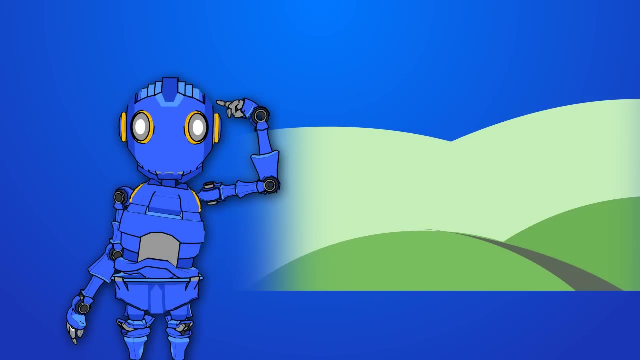 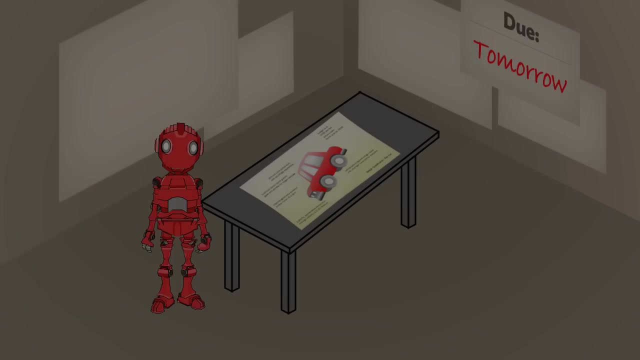 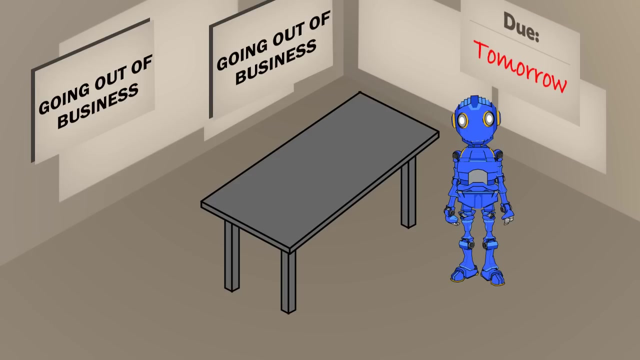 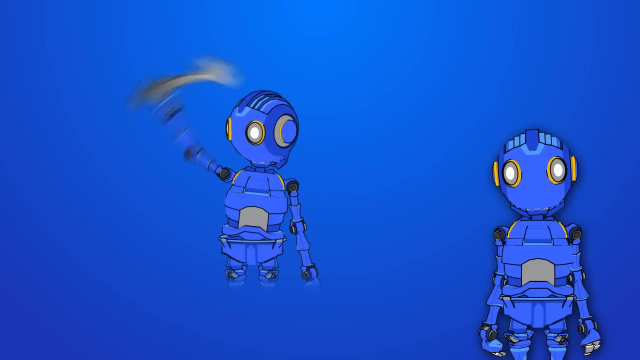 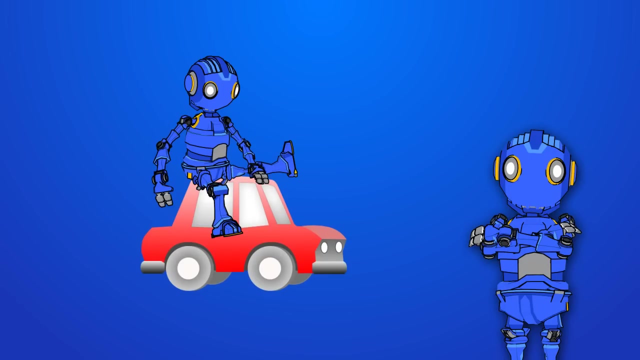 it first. Clearly, we didn't quite understand just who is going to be using it. you can avoid making the same mistakes. Engineering is about building solutions to problems, yes, but really solving them requires you to avoid these pitfalls. Engineering- a real solution to a real problem- includes the necessary research. 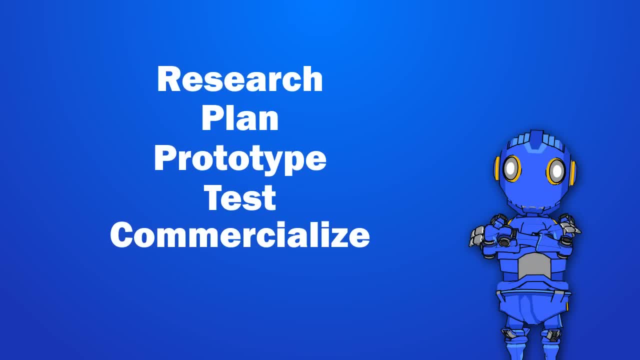 planning, prototyping, testing and commercialization processes to ensure real success.